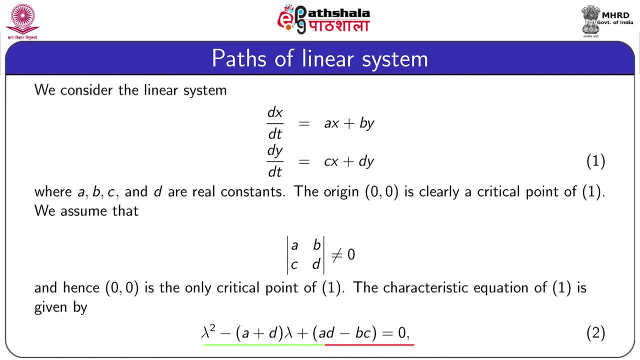 a plus d, The characteristic equation of 1 is given by equation 2.. Previously we have seen that if the characteristic equation given by 2 are real and negative, then we get a stable node. Here we will prove mathematically that actually we will get a stable node. 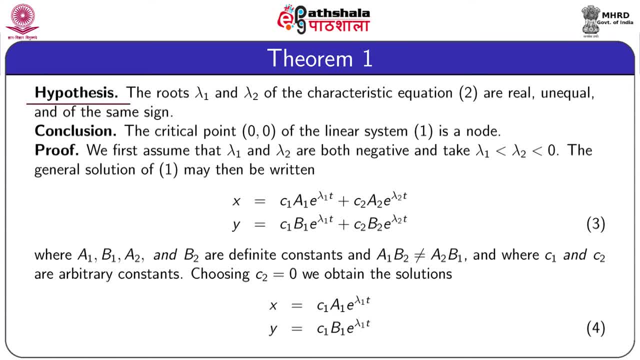 So the hypothesis is that if the roots lambda 1 and lambda 2 of the characteristic equation 2 are real, unequal and of the same sign, then we conclude that the critical point 0, 0 of linear system 1 is a node. We assume that lambda 1 and lambda 2 are both negative and we take lambda 1 less than lambda 2 and we come to the conclusion that lambda 2 is a node. We basically reduce whiteness of lambda 1 by and by juicy, theキ張 ax colon, And that means that the starting pointakof the linear system is a node. Here lambda 1 is equal to. 0 for kx and lambda 2 is equal to kx, d times lambda raise to k. which particular point bigger than indefinite? which particular full interval which means lambda k, the unit, which is meaning that lambda 1 and lambda 2 are indeed negative. So here we points in an answer to the healthy equation 2 and: 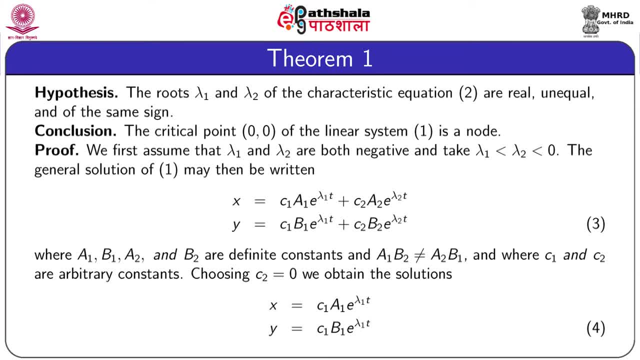 than lambda 2 less than 0.. Now the general solution of the linear system. 1 may be written as: x equal to c1 a1 e to the power lambda 1 t plus c2 a2 e to the power lambda 2 t. and. 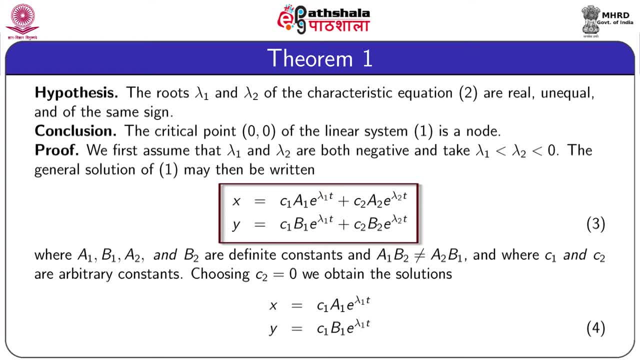 y equal to c1, b1. e to the power lambda 1- t plus c2, b2. e to the power lambda 2- t, where a1, b1 and a2- b2 are definite constants, provided a1- b2 is not equal to a2, b1 and c1 and c2. 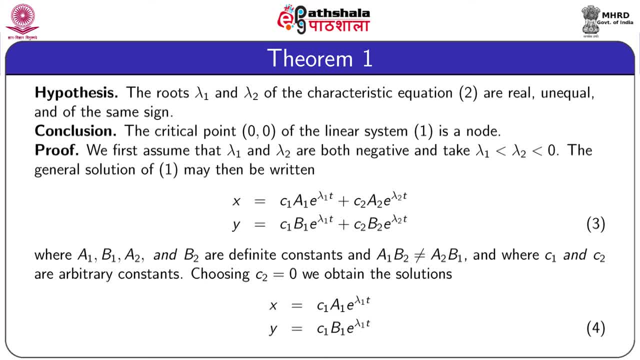 are arbitrary constants. Now, if we choose c2 equal to 0.. 0 and substitute it in equation number 3, we will get x equal to c1 a1- e to the power lambda 1 t, and y equal to c1 b1- e to the power lambda 1 t, which we name as equation 4.. 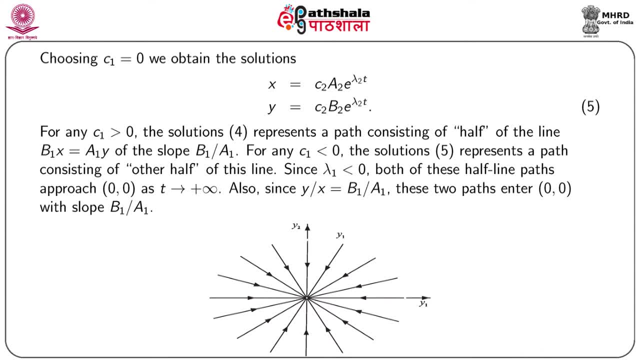 Similarly, choosing c1 equal to 0, we will obtain x equal to c2, b2, e to the power lambda 2 t, y equal to c2, b2, e to the power lambda 2 t given by equation 5.. Now for any c1 positive. the solution 4 represents a path consists of half of the line b1. x is: 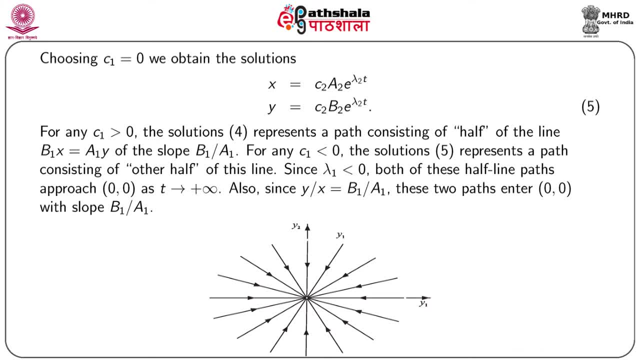 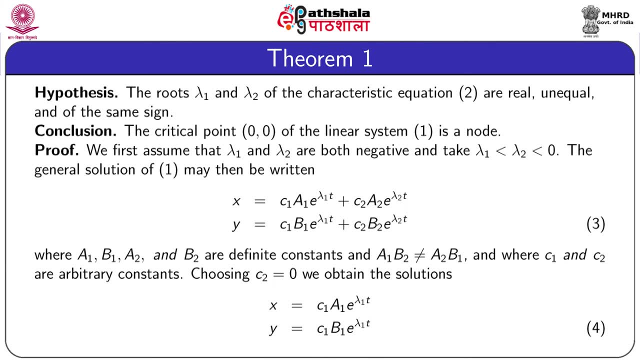 equal to a1. y of the slope b1 by a1.. The meaning of this is here: if we divide this, we will be getting x by y. this c1 and this c1 will cancel, and e to the power lambda 1 t. e to the power lambda 1 t will cancel. 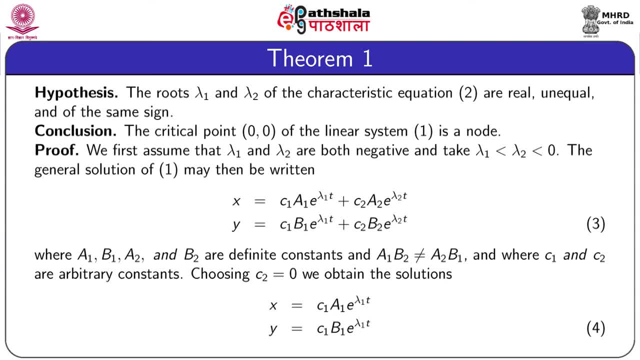 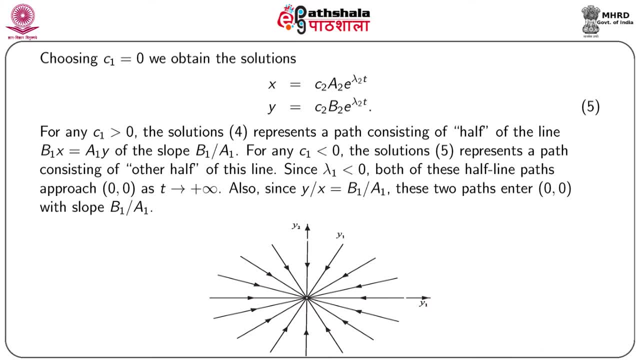 and you will be getting: y by x is equal to b1 by c1.. This is exactly shown here. that is, for any c1 positive. the solutions 4 will represent a path consisting of half of the line b1. x is equal to a1 by with slope b1 by a1.. 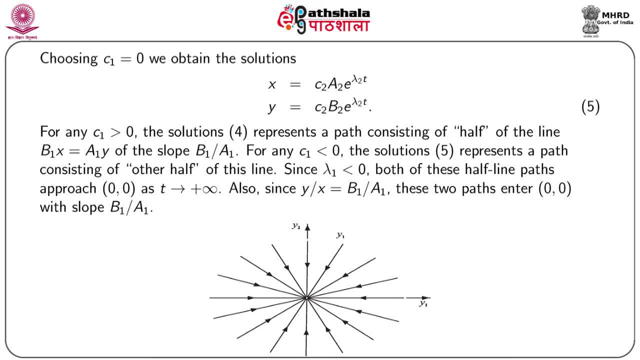 And for c1 less than 0, the solution 4 represent a path consisting of other half of the line And since lambda 1 is less than 0, both these half line paths approaches 0, 0 as t tends to plus infinity. 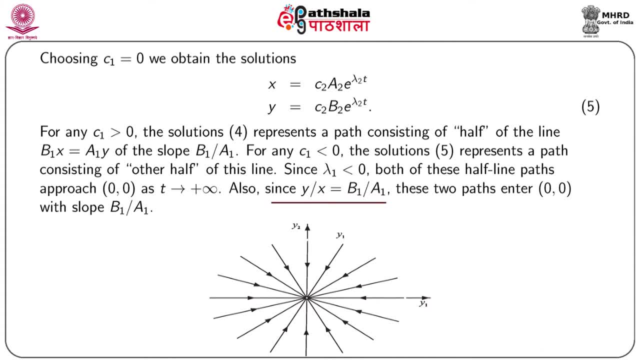 x is equal to b1 by a1, these two paths enter 0, 0 with slope b1 by a1.. Now if you look into the figure, you consider any one of this straight line. say this one. So the first. 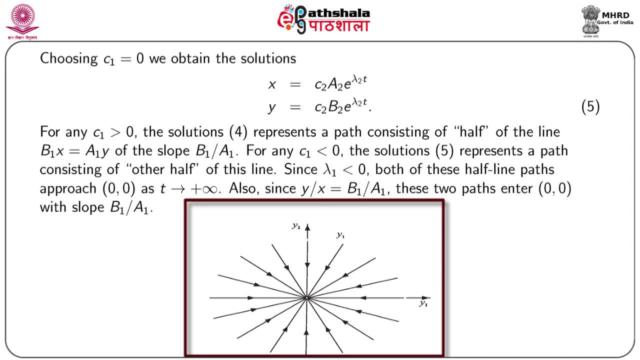 part says that if c1 is greater than 0, the solution represents a path consists of half of the line, b1 x equal to a1 y and let that half be this much, this half of the line. And if c1 is less than 0, the solution represents the other half. So, considering both, c1 greater 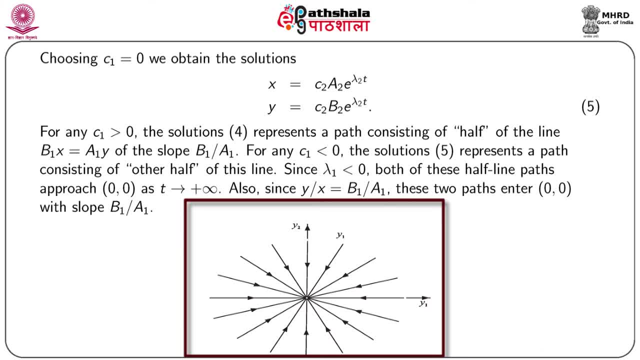 than 0 and c1 less than 0, we will get this full straight line. And since the straight line is of the form y equal to b1 by a1, x, that is y equal to m, x, where m the slope is b1 by a1, and we all know that it represents a straight line. 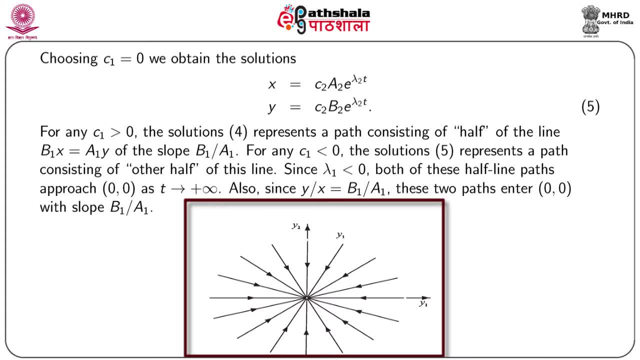 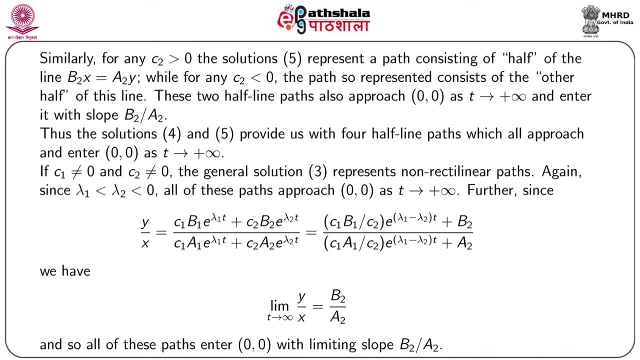 passing through the origin, And hence these two straight line will enter the origin with slope b1 by a1.. In the similar manner, for any c2 greater than 0, the solution 5 represents a path. This path consists of half of the line b2. x is equal to a2- y, while for any c2 less, 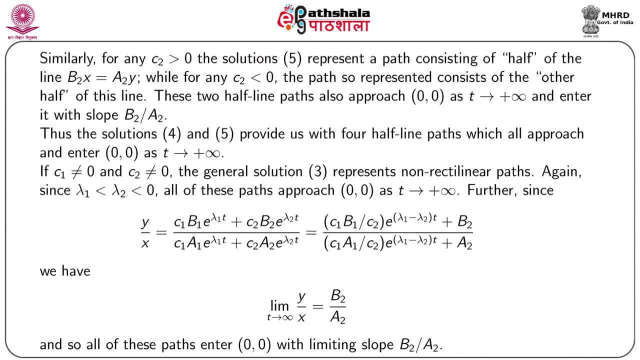 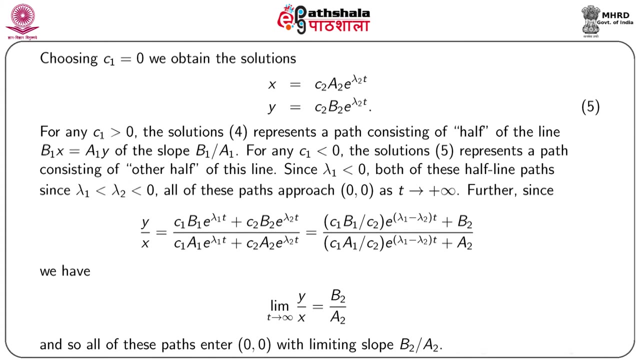 than 0,. the path so represented consists of the other half of this line And these two half line paths also approach 0: 0, as t tends to plus infinity and enters it with a slope b2 by a2.. This means that if we again consider this figure, that if we consider this as the line, 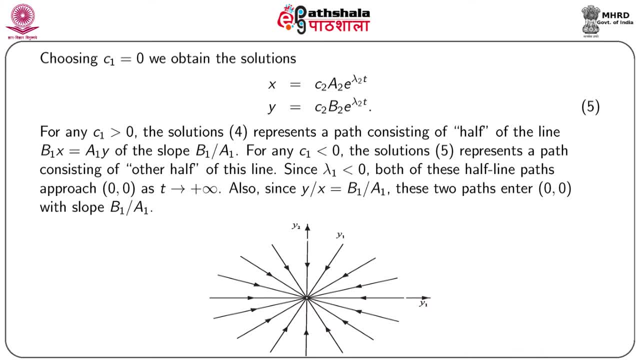 b2 x is equal to a2- y, then for c2 positive, let it represent this particular straight line and for c2 negative, it represents this particular straight line. And both of them, And since it is a straight line passing through the origin, both these half lines will enter. 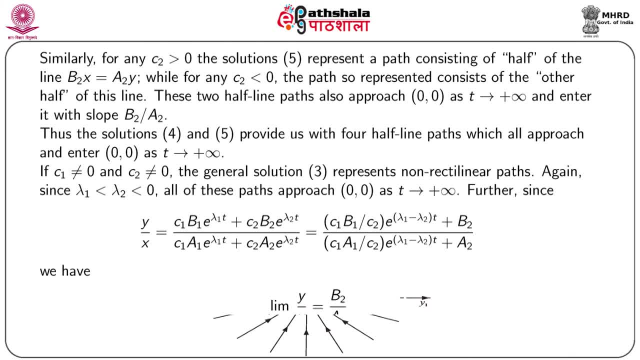 the point. Thus the solutions 4 and 5, it provides us with four half line paths which approaches and enters, as t tends to plus infinity. Now let us consider the case when neither c1 nor c2 is equal to 0. There is c1 not equal. 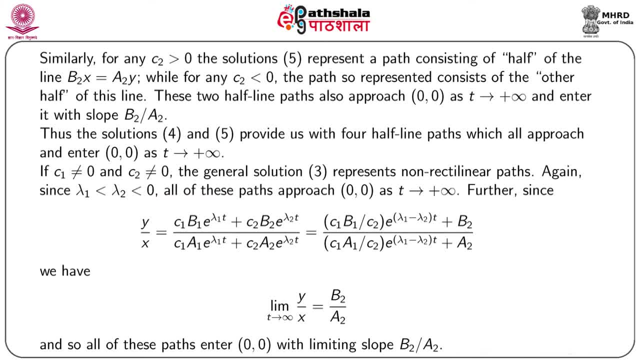 to 0 and c2 not equal to 0. And then the general solution 3 represents a non-rectilinear paths. We have already assumed that lambda 1 is less than lambda 2 is less than 0. And all these paths will approach 0- 0 as t tends to plus infinity. 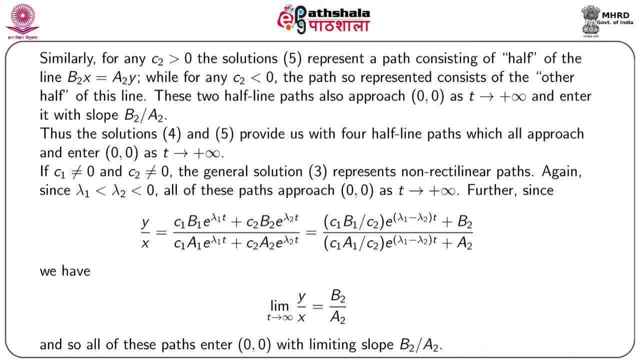 Further, if we calculate this ratio y by x, which is equal to c1, b1, e to the power lambda 1 t plus c2, b2 e to the power lambda 2 t divided by c1, a1 e to the power lambda 1 t plus c2. 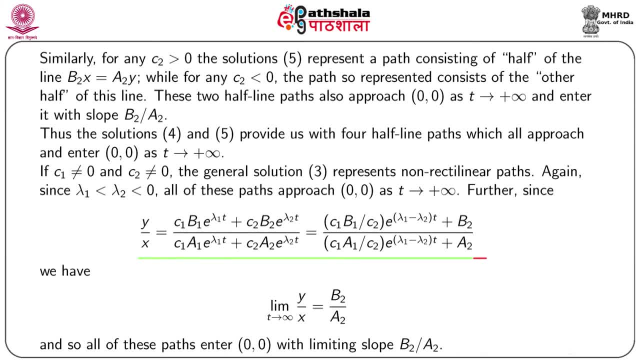 a2 e to the power lambda 2 t, We will be getting c1 b1 by c2 e to the power lambda 1 minus lambda 2 into t, and likewise the denominator, As t tends to infinity. we can see: lambda 1 minus lambda 2 is less than. 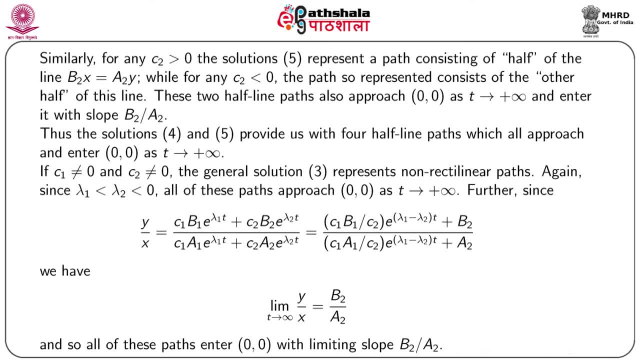 0 and this whole term will tend to 0.. This all term also tends to 0, as t tends to plus infinity And hence we will have limit. t tends to plus infinity. y by x is equal to b2 by a2.. And 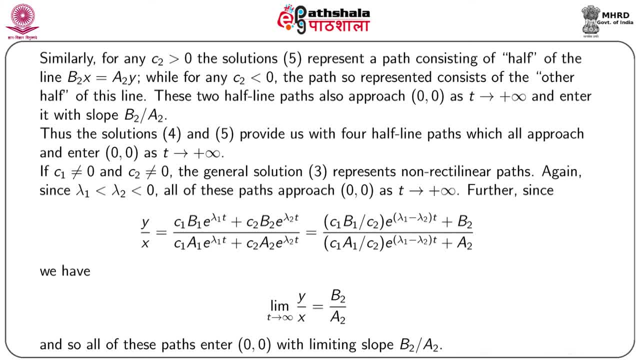 so by definition, these paths will enter 0: 0 with a limiting slope, b2 by a2.. And hence we get that if both the roots lambda 1 and lambda 2 are real, unequal and less than 0, then the given system will represent a node at the origin And in this case it is a stable. 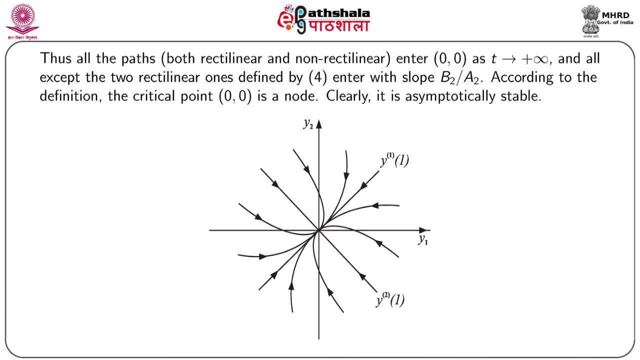 node. Thus we conclude that all the paths, both rectilinear and non-rectilinear, they enter 0, 0 as t tends to plus infinity, and all except two rectilinear ones enter with slope lambda, Still with slope b2 by a2.. And according to the definition, the critical point is: 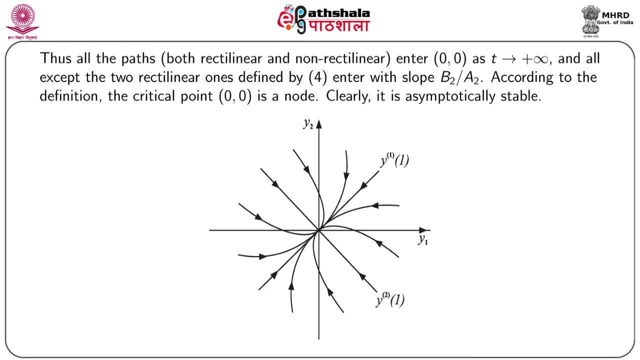 the node and clearly it is asymptotically stable. Now if lambda 1 and lambda, Now if lambda 1 and lambda 2 are both positive and we take lambda 1 greater than lambda 2 greater than 0, we see that the general solution of 1 is: 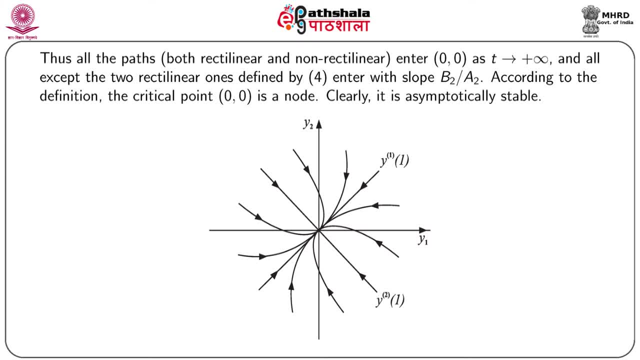 still in the form 3.. And the particular solution of the form 4 and 5 still exists And is really unequal and will depend on ourlebr controlar. ourb gemacht, Hi French. Well, thank you very much. 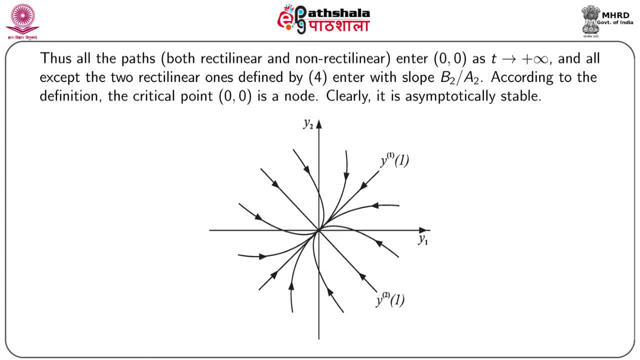 The situation is same as before, except the all the paths approach and enter zero, zero, as t tends to minus, infinity. The critical point: zero, zero is still a node, but it is in this case it is unstable. and please note, since the node is unstable, all the arrows. 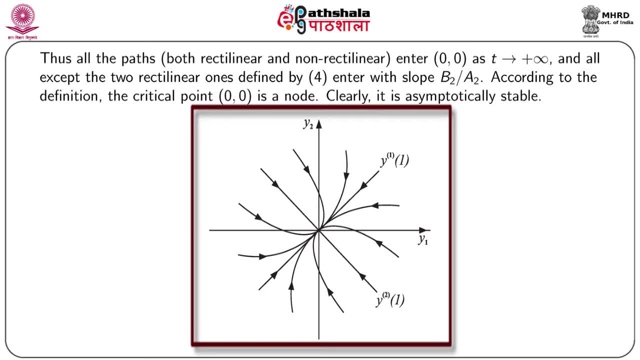 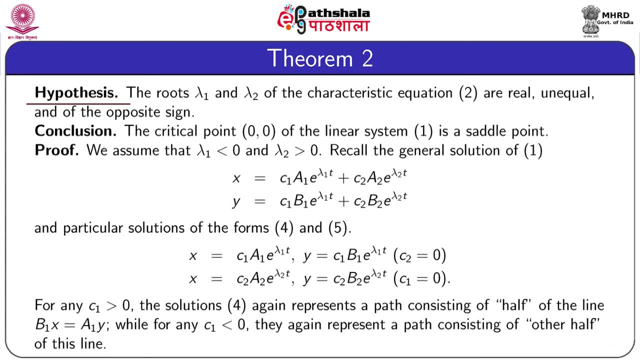 here are moving away from the origin In our second theorem. our hypothesis is that the roots lambda 1 and lambda 2 of the characteristic equation 2 are real, unequal and of the opposite sign. The critical points in this case is a saddle point and since they are of opposite sign, we assume that let lambda 1 is less than 0 and lambda 2 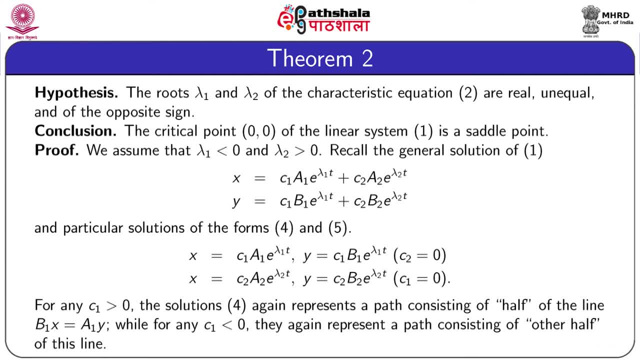 is greater than 0.. Our general solution of 1 is taken as: x is equal to c1, a1, e to the power lambda 1, t plus c2, a2, e to the power lambda 2 t and y equal to c1, b1, e to the power lambda 1 t plus c2. 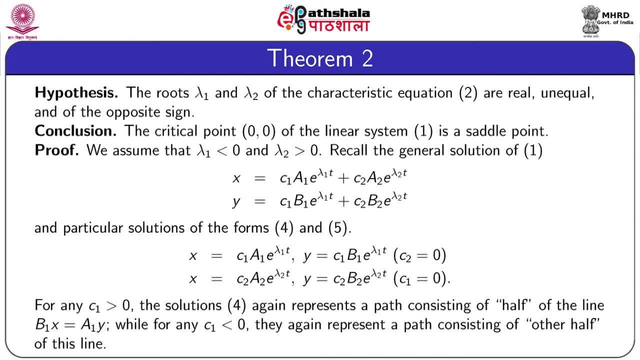 b2 e to the power lambda 2 t, And the particular solutions are of the form 4,, b1, e to the power lambda 1 t plus c2, b2, e to the power lambda 2 t, And the particular solutions are of the form 4 and 5, which is x equal to c1, a1, e to the power lambda. 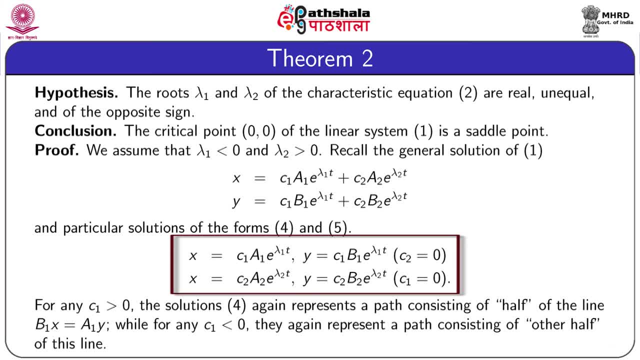 1 t. y equal to c1, b1. e to the power lambda 1 t which is obtained by putting c2 equal to 0. And when we put c1 equal to 0, we will get. x is equal to c2. a2. e to the power lambda 2 t. 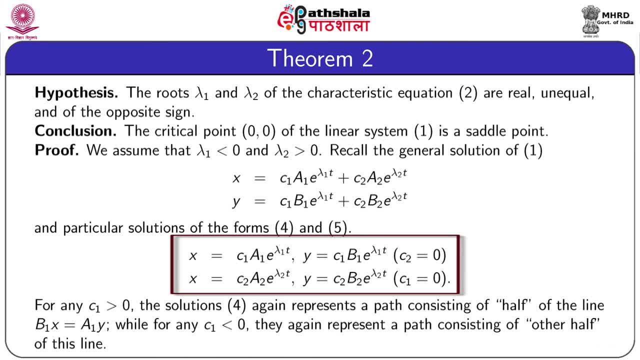 y equal to c2, b2, e to the power lambda, 2, t. Here a1, b1, a2, b2 are definite constants and c1 and c2 are arbitrary constants. So, like before, if c1 is greater than 0, the solution 4 represents a path consisting of: 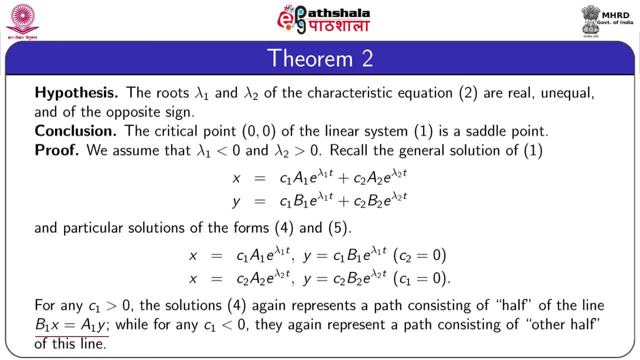 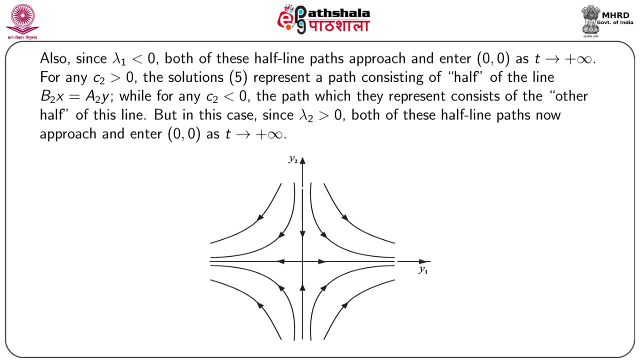 half of the line. b1- x is equal to a1- y, while for c1 less than 0, they will again represent a path consist of the other half of the line. So in this case, since lambda 1 is greater than 0 and lambda 1 is negative, we will get this as a half of the line which is approaching. 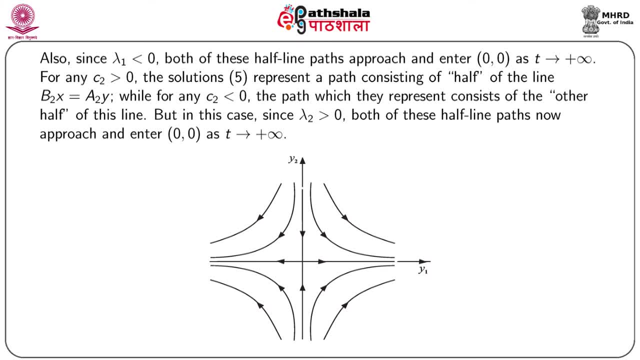 the point 0: 0, and this as another half of the line which is again approaching 0: 0.. So since lambda 1 is negative, both these half lines approach 0: 0 and enter 0: 0 as t tends to plus infinity. Now, for any c2 positive, the solution 5 represents a path consists of half. 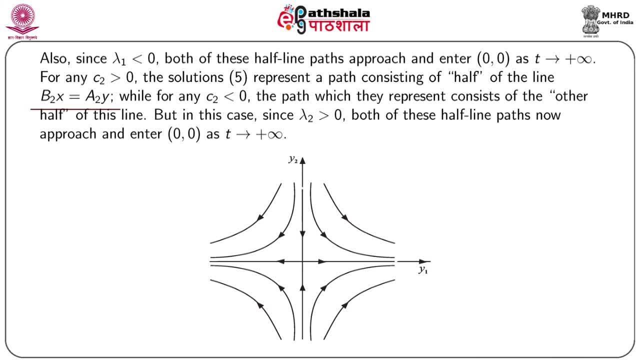 of the line b2 x equal to a2 y, while for any c2 less than 0 the path represents consist of other half of this line. But since in this case lambda 2 is greater than 0, both of these half line paths now approach and enters 0, 0 as t tends to minus infinity and hence in. 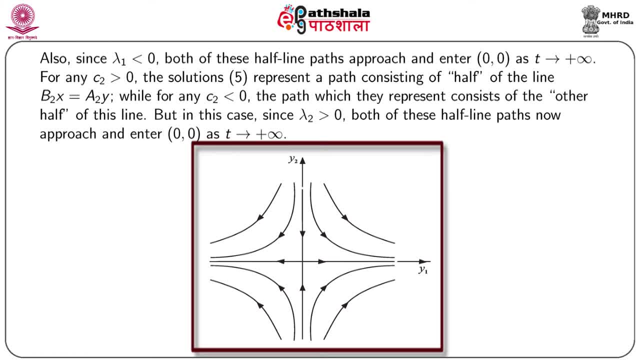 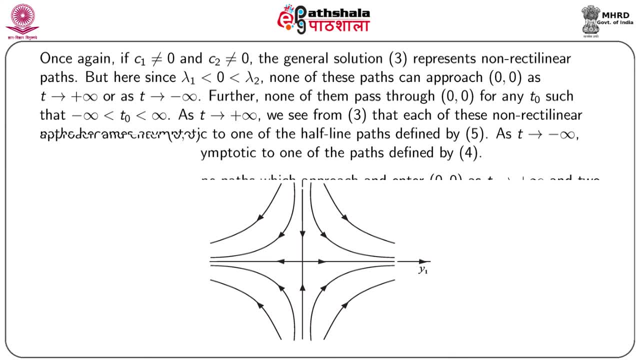 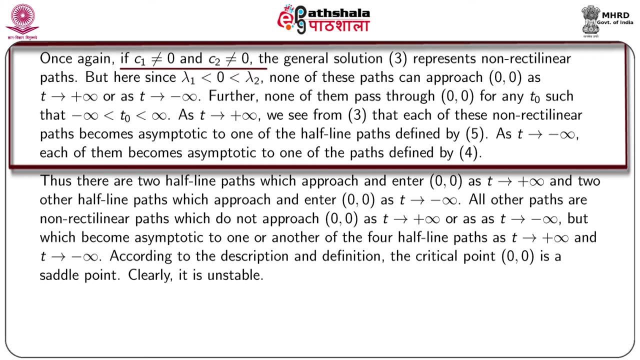 this case we will get this straight line where it is greater than 0.. moving away from the origin, And if c1 not equal to 0 and c2 not equal to 0, the general solution 3 represents a non-rectilinear paths And since lambda 1 is less than 0 and lambda 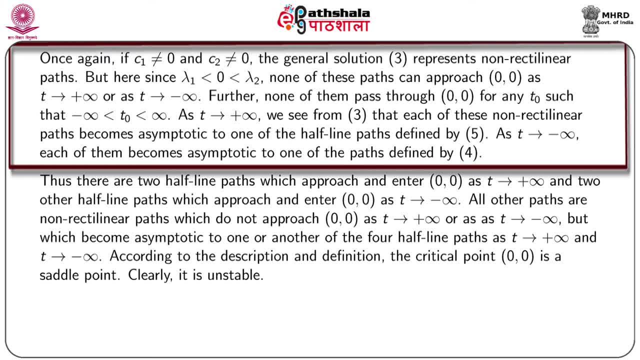 2 is greater than 0,. none of this path can approach 0, 0 as t tends to plus infinity or as t tends to minus infinity. Moreover, none of them pass through 0, 0 for any t0, such that minus infinity, less than t0, less than infinity. 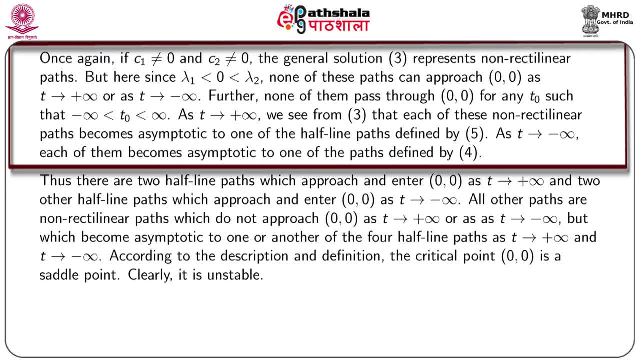 As t tends to plus infinity, we see from 3 that each of these non-rectilinear paths becomes asymptotic to one of the half-line paths defined by 5.. And as t tends to minus infinity, we see from i to 1, each of them becomes asymptotic to one of the paths defined by 4.. 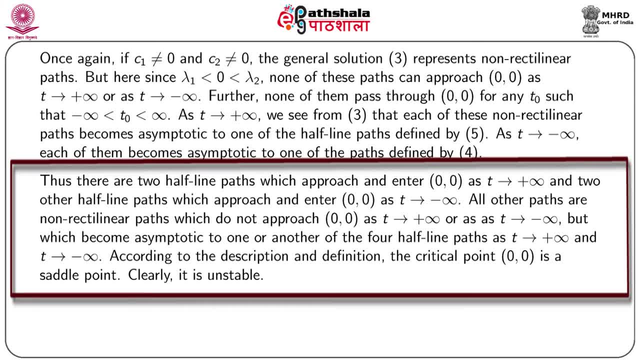 Therefore, there are two half-line paths which approach and enter 0, 0 as t tends to plus infinity, and two half-line paths which approach and enter 0, 0 as t tends to minus infinity. All other paths are non-rectilinear paths which do not approach 0, 0 as t tends to plus infinity. 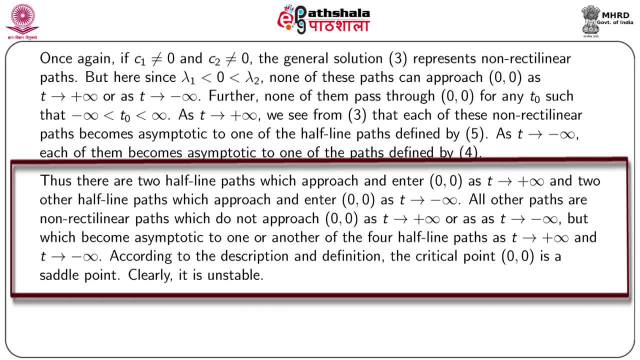 as t tends to minus infinity. But it will become asymptotic to one or another of the four half line paths, as t tends to plus infinity or as t tends to minus infinity, And hence, by definition, the critical point is a saddle point and clearly it is unstable. 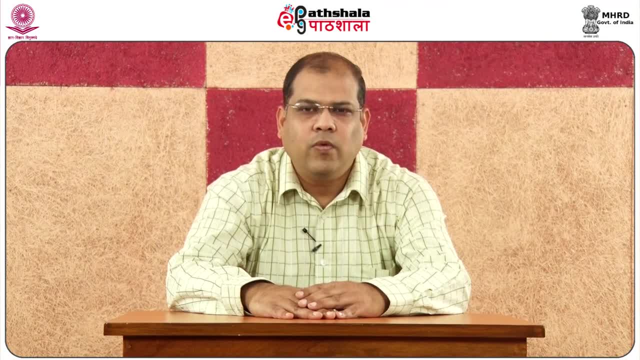 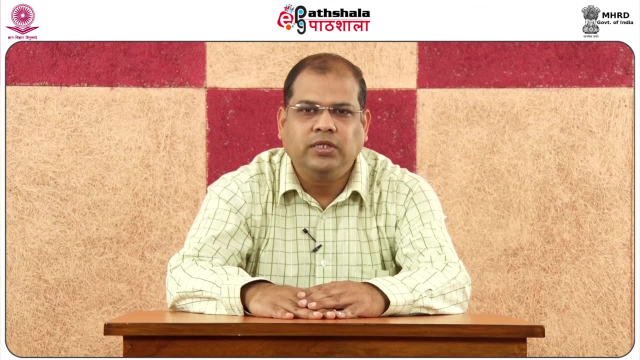 We have just looked into the system of linear equations, where we have taken two linear equations and we have proved that if the roots are real and negative, then it will represent a node. We will now look into the generalized system of linear equations and look into its stability. 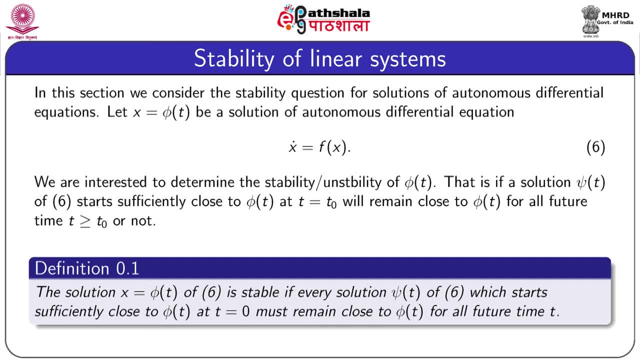 Here we consider the stability question for the solution of autonomous differential equation. Let x equal to phi t be a solution of the autonomous differential equation of the form x dot, which is d x. Let x equal to phi t be a solution of the autonomous differential equation of the form x dot, which is d x. 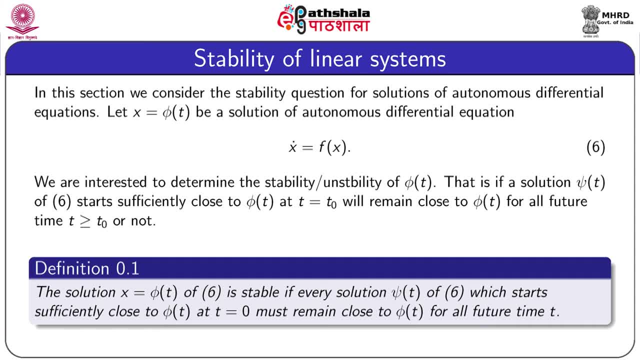 We are interested in determining whether phi t is a stable or unstable solution, That is, whether every solution, psi t of 6, which starts sufficiently close to phi t at t equal to t 0, must remain close to phi t for all future time. t greater or equal to: 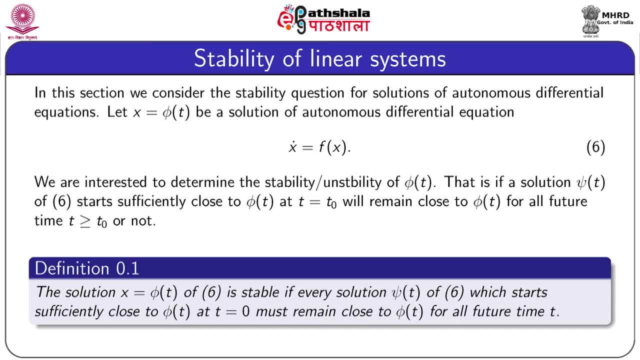 t 0.. Now the definition: the solution x equal to phi t of 6 is stable if every solution psi t of 6 which starts sufficiently close to phi t at t equal to 0 must remain close to phi t for all future time. t. 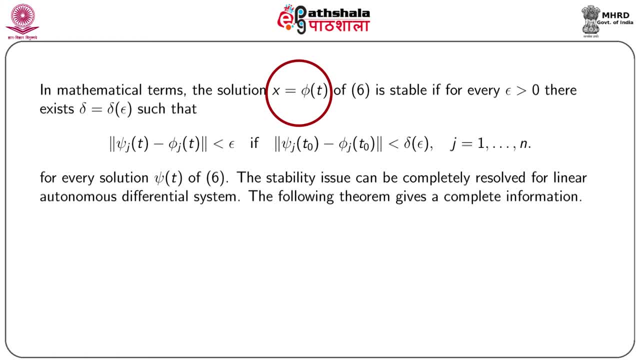 In mathematical terms, the solution x equal to phi t of 6 is stable if for every epsilon positive there exist a delta which depends on epsilon, such that norm of psi j t minus phi j t is less than epsilon. if norm of phi j t0 minus psi j t0 is less than delta which 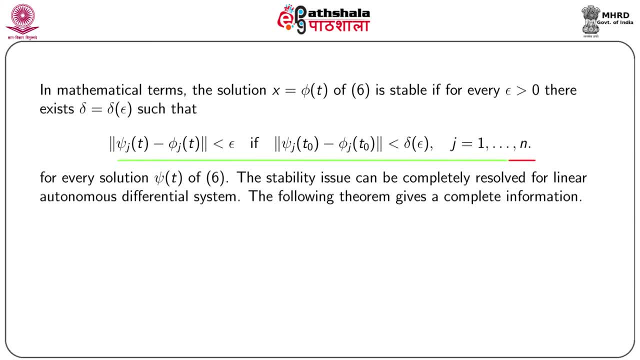 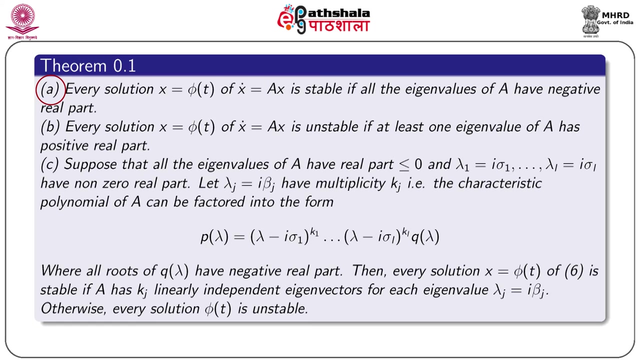 is a function of epsilon: j equal to 1 to dot dot n for every solution, psi t of 6.. The stability issue can be completely resolved for linear, autonomous differential equation and the following theorem gives the complete information: Every solution x equal to phi t of x, dot equal to Ax is stable if 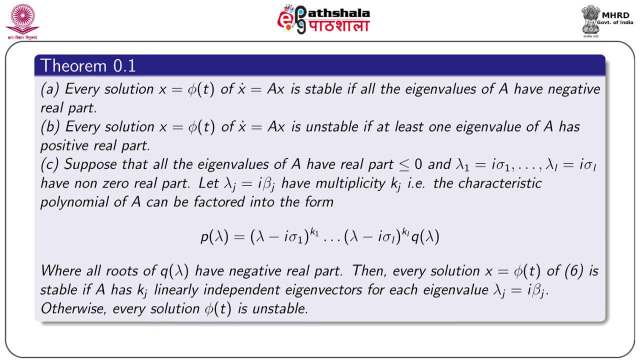 This means Here I have go ahead. take only this hypothesis. Here I have taken a very previous definition here I have talked to you earlier, and this was applied to Parkinson's and T cell physics, which I cant forget here today. Then for me the possible binary is very simple here. 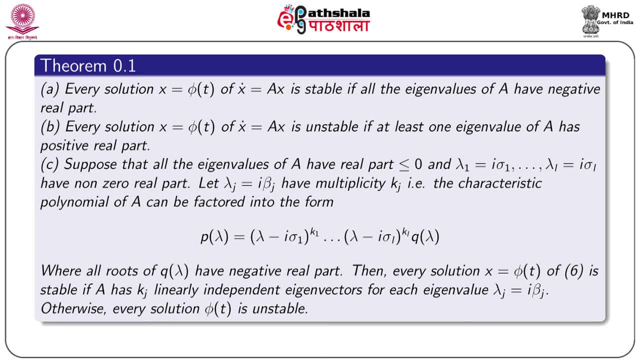 dot dot. lambda l equal to i sigma l have non-zero real part. Let. lambda j is equal to i sigma j have multiplicity K. j, that is the characteristic polynomial of A, can be factored into the form P: lambda is equal to lambda minus i sigma 1 to the. 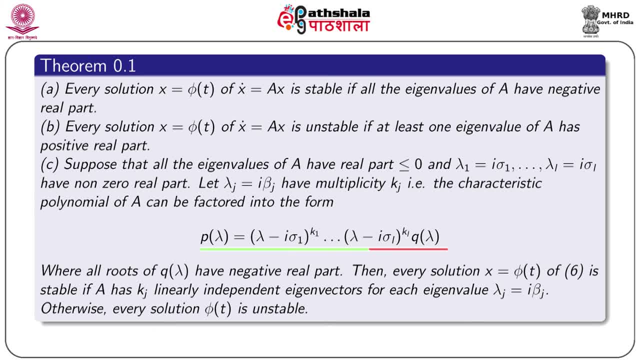 power K 1 dot dot lambda minus i sigma l to the power K l Q lambda. where all the roots of Q lambda have negative real part, Then every solution x equal to phi t of 6 is stable. if K has K, j linearly independent eigenvectors for each eigenvalue lambda j equal to i sigma. 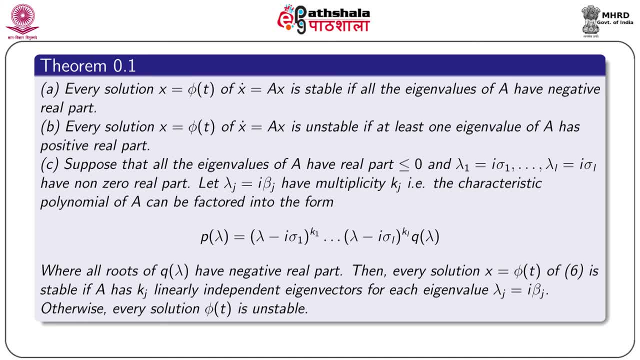 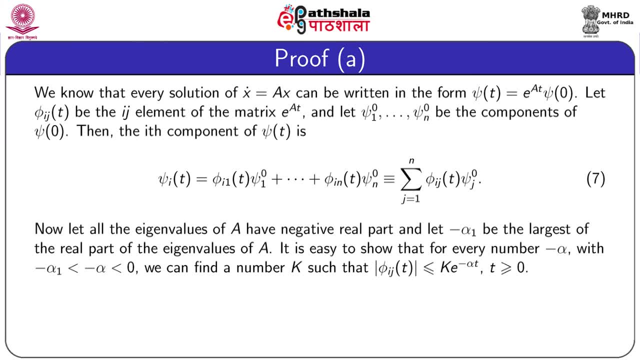 j. Otherwise K j is independent. Every solution phi t is unstable. The proof of the first part: we know that every solution x dot is equal to A. x can be written in the form: psi t is equal to e, to the power A t, psi 0.. Let phi i j t be the. 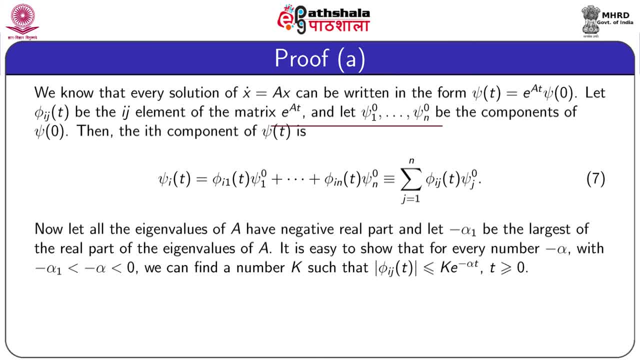 i, j th element of the matrix e to the power A, t, and let phi 1, 0, phi 2, 0, dot dot, psi n, 0 be the components of psi 0. Then the i th component of psi is psi i t is equal to phi. 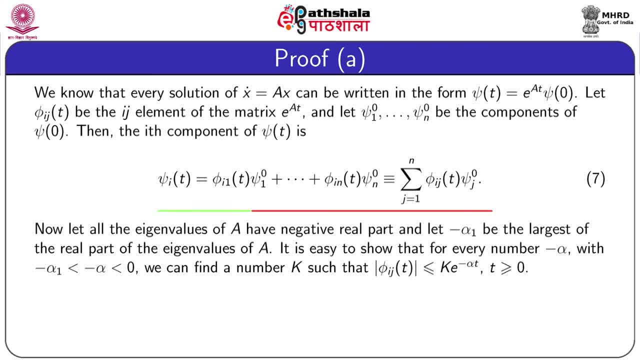 i 1 t psi 1 0 plus dot dot plus phi i n t psi 1 0 plus dot dot plus phi i n t psi 1, 0, which is equivalent to summation j equal to 1 to n. phi i j t psi j 0, given by equation. 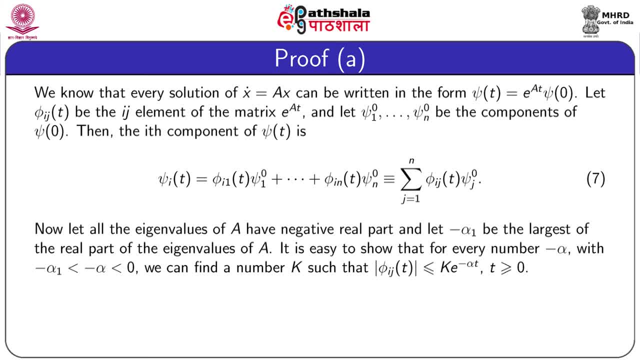 7. Now let all the eigenvalues of A have negative real part and let minus alpha 1 be the largest of the real part of the eigenvalues of A. It is easy to show that for every number minus alpha, with minus alpha 1, less than minus alpha, less than 0, we can find a number capital. 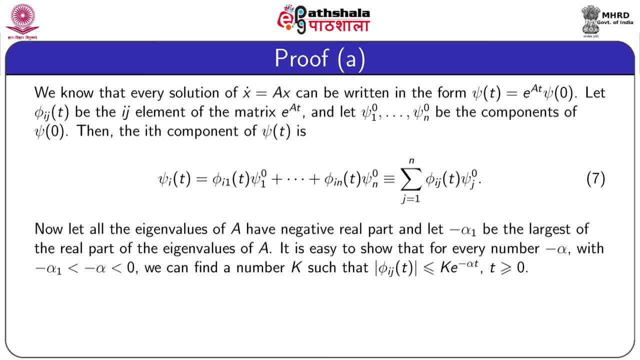 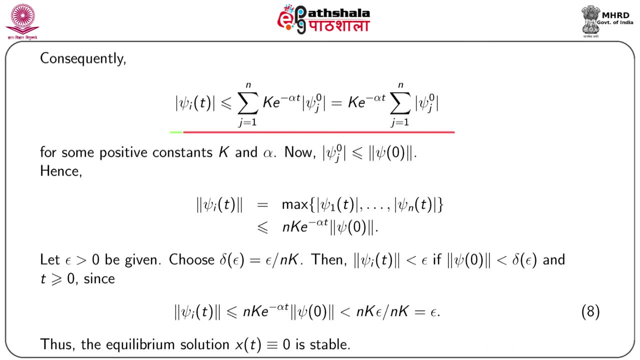 K, such that mod of phi i j t is less or equal to K times e to the power minus alpha t, where t is greater or equal to 0.. Consequently, mod of psi i t is less or equal to summation j or equal to summation j, equal to 1 to n k e to the power minus alpha t. mod of psi j. 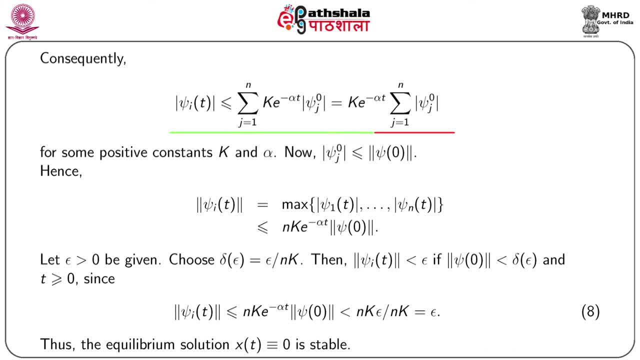 0, which is equal to k, e to the power minus alpha t. summation: j equal to 1 to n. mod of psi j 0: for some positive constants, k and alpha, Now, mod of psi j 0 is less or equal to norm of psi 0 and hence norm of psi i t is equal. 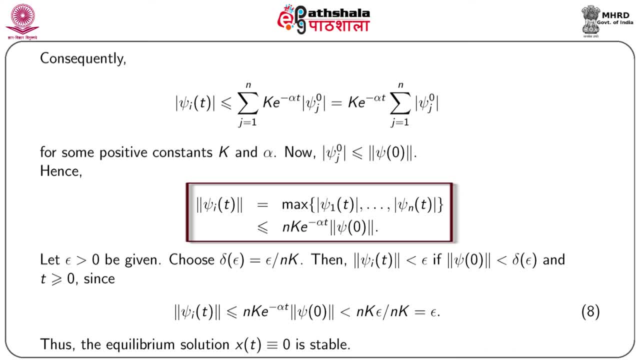 to maximum of mod of psi 1 t. mod of psi 2 t. dot dot. mod of psi n t which is less or equal to n k e to the power minus alpha t norm of psi 0.. Let epsilon greater than 0 be given and we choose delta. 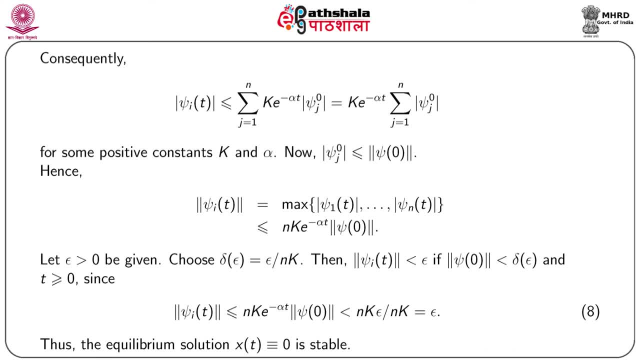 So norm of psi i t is equal to epsilon divided by n- k. then norm of psi i t is less or equal to epsilon if norm of psi 0 is less than delta and t greater equal to 0.. Since norm of psi i t is less or equal to n k e to the power minus alpha t norm of psi 0, which is less, 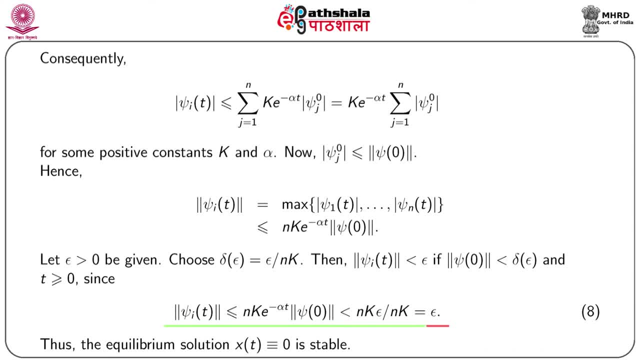 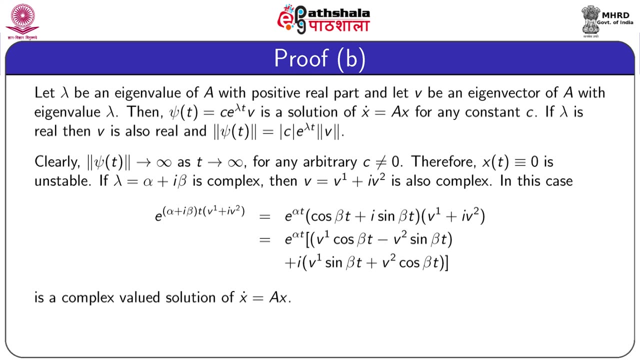 than n k epsilon. divided by n k equal to epsilon, The equilibrium solution x t equal to 0 is stable. For the second part of the proof, let lambda be an eigenvalue of A with positive real part and let V be an eigenvector of A with eigenvalue lambda. Then psi t is equal to c, e to the. 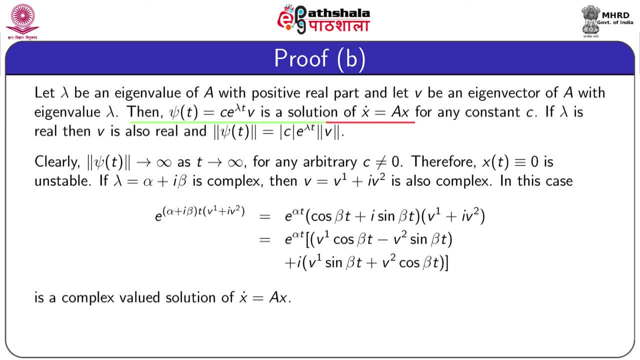 power, lambda, t, v. The equilibrium solution, gospel root i, 0, is a solution of x, dot equal to A, x for any constant c. If lambda is real, then V is also real and norm of psi t is equal to mod c, e to the power. 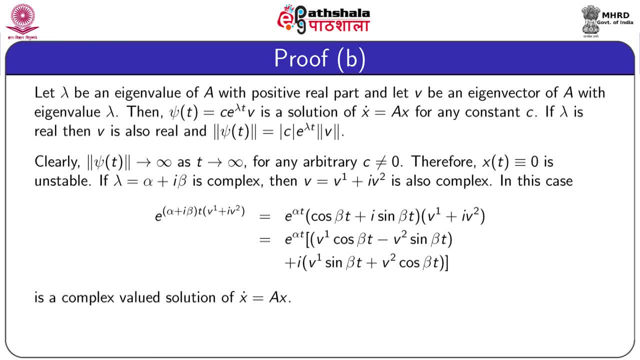 lambda t, norm of V, Clearly norm of psi, t tends to infinite, as t tends to infinite for any arbitrary c not equal to 0. Therefore, x dot equal to A, x will be equal to 0. So x t equal to 0 is unstable. And if lambda equal to alpha plus i, beta, be complex, let 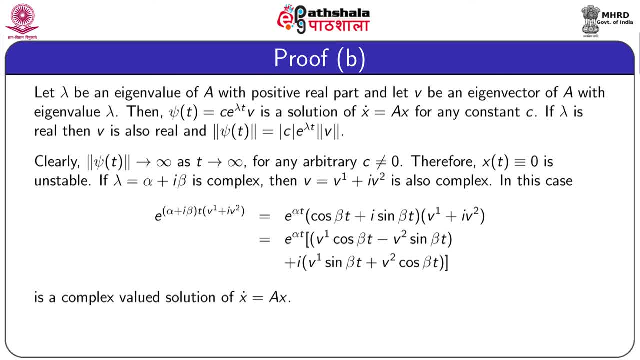 v equal to v1 plus i. v2 is also complex, In this case e to the power alpha plus i beta t into v1 plus i. v2 is equal to e to the power alpha t, cos beta t plus i, sin beta t. 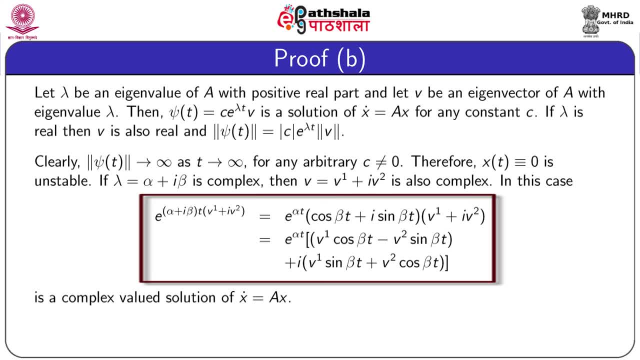 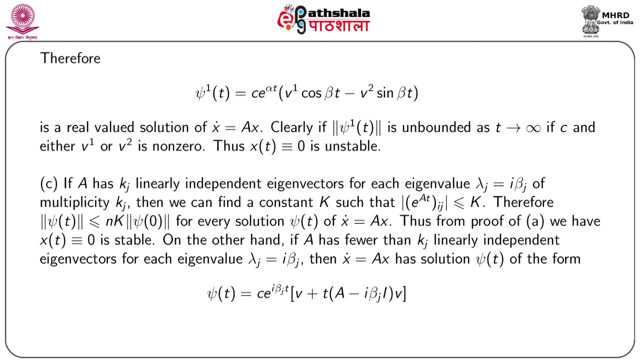 v1 plus i v2, which can be written as e to the power alpha t: v1 cos beta t minus v2 sin beta t plus i times v1 sin beta t plus v2 cos beta t is a complex value solution of x dot equal to Ax. Therefore psi 1 t is equal to c. e to the power alpha t: v1 cos beta t. 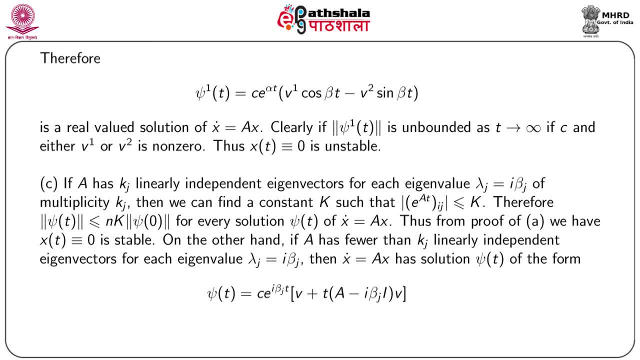 minus v2, sin beta t is a real valued solution of x dot equal to Ax. Clearly, if norm of psi 1, t is unbounded, as t tends to infinity if c and either v1 or v2 is nonzero. thus x t equal to 0 is unstable. And from the proof of c, if a has k equal to, 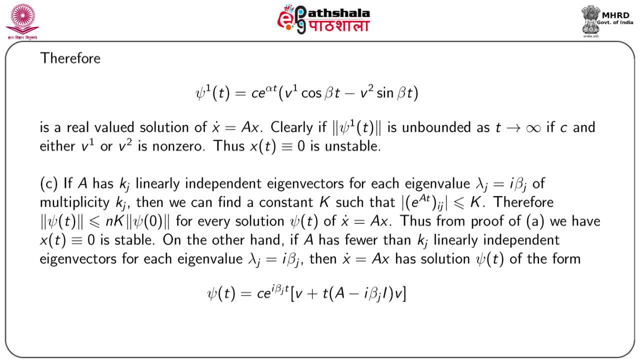 kj, linearly independent eigenvectors for each eigenvalue, lambda j equal to i, sigma j of multiplicity kj. then we can find a constant k such that mod of e to the power a, t, ij is less or equal to k. Therefore, norm of psi t is less or equal to nk. norm of psi 0 for. 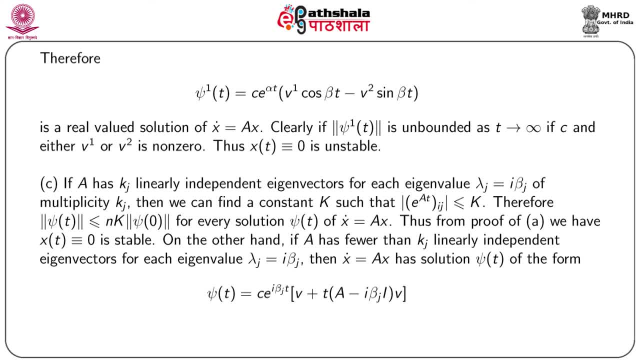 every solution. Thus from the proof of a we have x. t equal to 0- is stable. On the other hand, if a has fewer than kj linearly independent eigenvectors, for all eigenvalue, lambda j equal to i, sigma j, then x dot equal to Ax has the solution psi t. of the form psi t is equal to sigma. 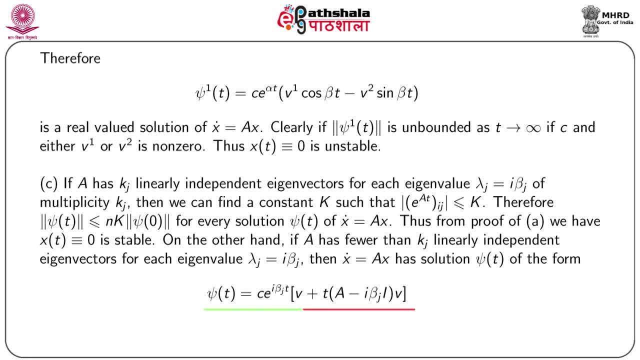 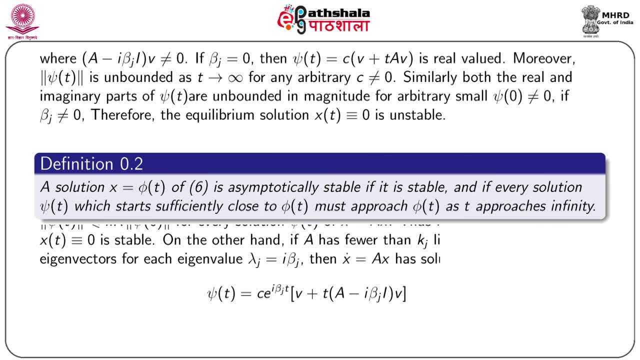 j. Similarly, from the proof of c e to the power i sigma j t v plus t times a minus i sigma j i into v, where a minus i sigma j i into v not equal to 0.. If sigma j equal to 0, then: 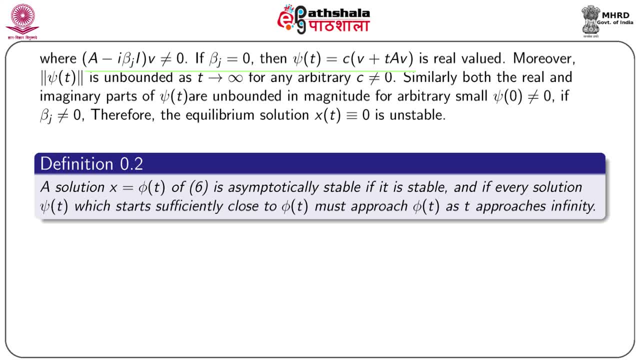 psi t is equal to c, v plus t, av is real valued. Moreover, norm of psi t is unbounded as a real valued solution And from example 0.2, it gives a solution: x equal to phi t of 6 is asymptotically stable. 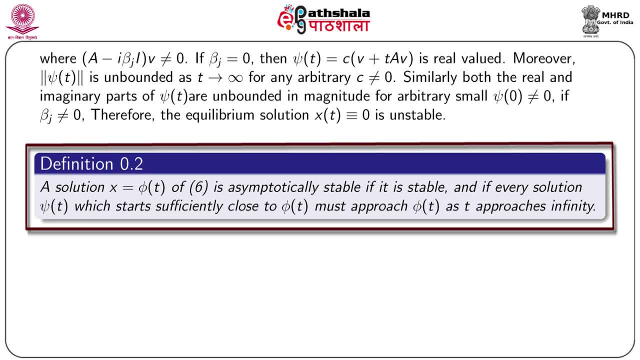 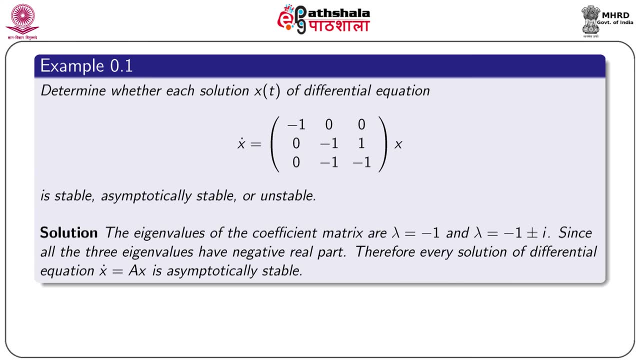 if it is stable and if every solution, psi t which starts sufficiently close to phi t must approach phi t as t tends to infinity. Now let us consider the example where psi, where we have to check whether the system of the differential equation given by x dot. 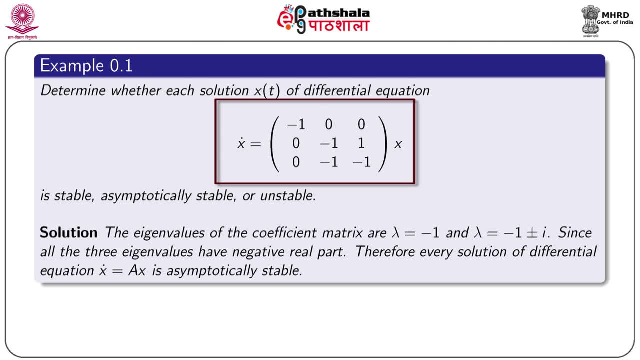 or dx. dt is equal to Ax, where A is minus 1, 0, 0, 0 minus 1, 1 and 0 minus 1 minus 1 is stable, asymptotically stable or unstable. Now we can easily find the eigenvalues of this coefficient. 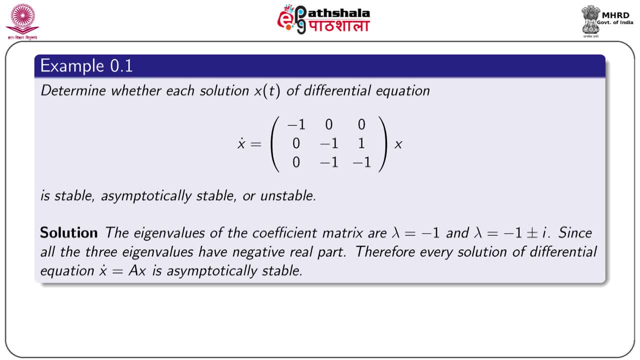 matrix from the definition mod of A minus lambda I is equal to 0. And if you solve that, we will get lambda equal to minus 1 and lambda equal to minus 1 plus minus I, Since all the three eigenvalues have negative real part. therefore, every solution of this differential